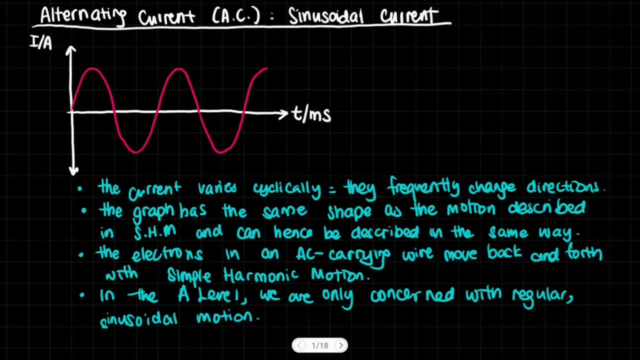 voltage, and we're going to talk about the power of alternating currents using the root mean squared of the alternating current as well as the alternating voltage values. so let's start. the first thing you need to know about these alternating currents is that they are sinusoidal currents, and that means that they have this if you graph them out with respect to time. this is: 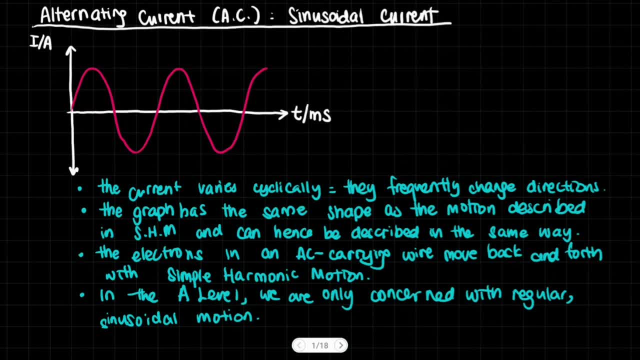 what turns out? it's a sine curve, and so you know. the definition of an alternating current is a current that goes back and forth, it changes direction regularly. it doesn't mean that it has to be this regular sinusoidal current. though it could be jerky, it could be erratic, it doesn't have. 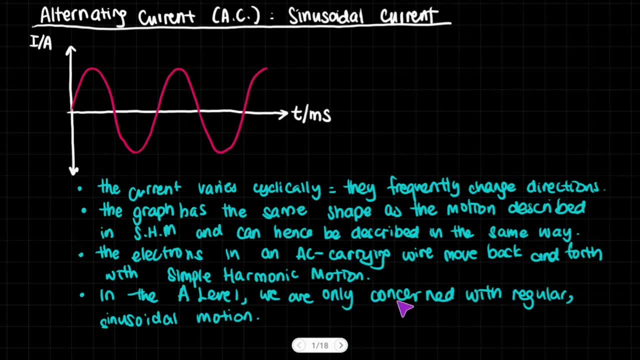 to be the smooth curve. however, in the a level, we are only concerned with regular sinusoidal motion. so think of this, at least at this level, the current has has a variation that's cyclical, so that means that they frequently change directions and it follows this type of motion. 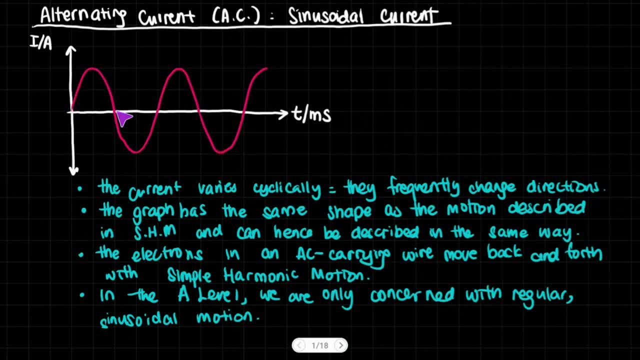 where it increases and then it slowly decreases, and then it changes direction, increases in magnitude, decreases in magnitude, changes direction, and that keeps going. now, this has to remind you of something: the graph has the same shape as the motion described in simple harmonic motion and hence can be described in the same way. something that's very common in physics as well as engineering is 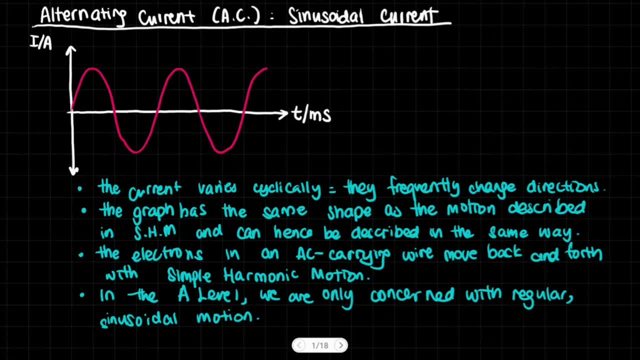 when you find that a certain phenomena or a certain phenomenon has this some sort of formula and you know another phenomenon that has the exact same formula or it has the same form, then you can take whatever results, whatever experiments has happened in that other phenomenon, and you can. 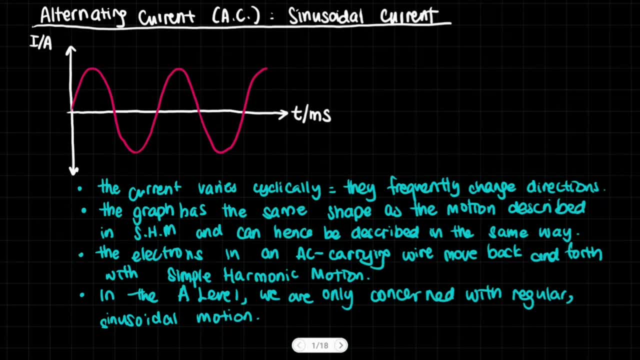 also apply to this one. let's give it a try. let's give you an example. for instance, the force of attraction between two charges is- this is a constant of proportionality- and then we have charge one, charge two divided by separation. squared. however, the force of attraction between two masses, that's gravitational attraction, is gmm over r. 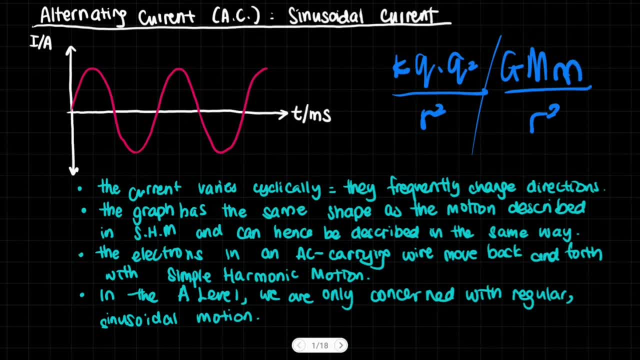 squared, so the form of these two is the same, and this is why we have a constant of proportionality. here's another truth. look, you have to look at the initial Noise over here and you'll see how the forcing of these two charges. questo is pretty happen because we're not have 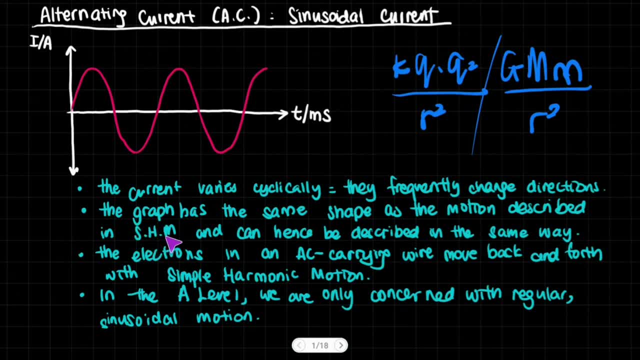 the same force between those a or b. this is the same resistivity as from a at likes to say the same force between them, because the thrust force is the force of that and because the force of Ray with Cheese we're also going to be speaking about a dependent force- is. 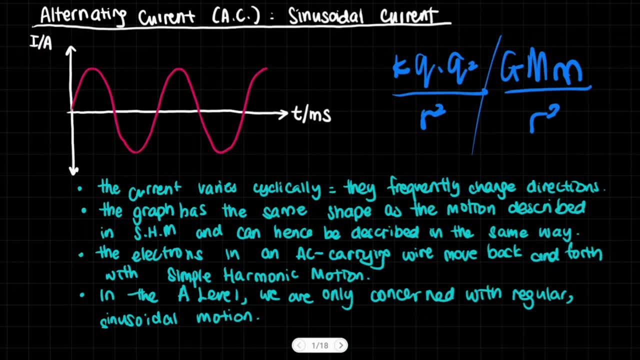 sense, if you look at the graph now- the the current here, that is kind of you can think of it as the velocity graph of an electron right, because it's the rate of flow of charge. so you can kind of think of this as a velocity graph. it starts: 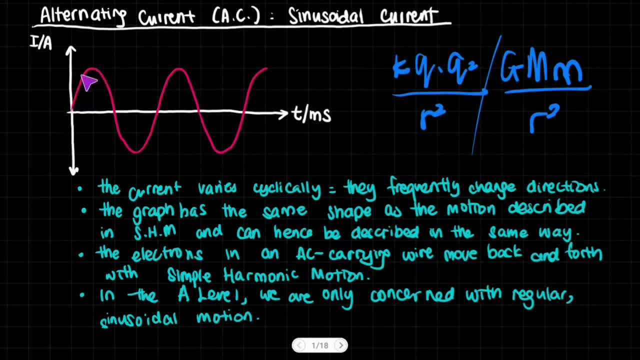 out at zero and then it accelerates towards a peak and then it goes down again and then it changes direction after it comes to momentary stop and then it becomes very, very fast and then it slows down again, changes direction, etc. that is what simple, harmonic motion is: if you have an object in simple 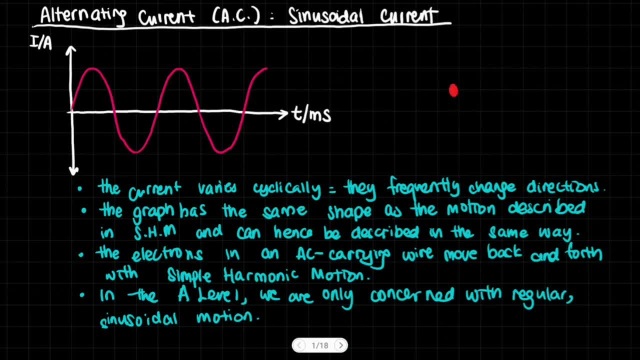 harmonic motion. what it will do is that it has an equilibrium position at which the velocity is maximum, and then you accelerate, you. you move very quickly and you're decelerating and you slow down at the end and you momentarily stop, and then you change direction and you accelerate again, and then you. 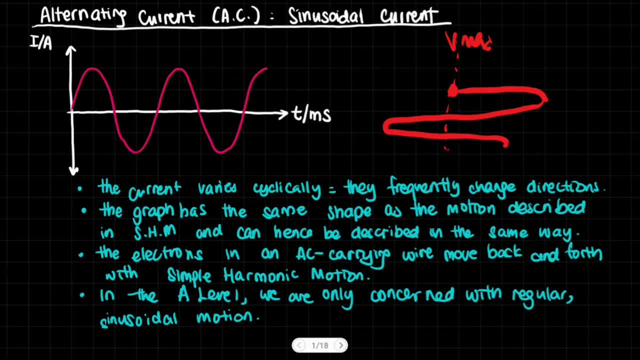 decelerate and you move very quickly and you change direction and then you slow down, you stop, and then you, you know that's, that's how it goes right. and then the definition for simple harmonic motion is that the acceleration of the object is directly proportional to the 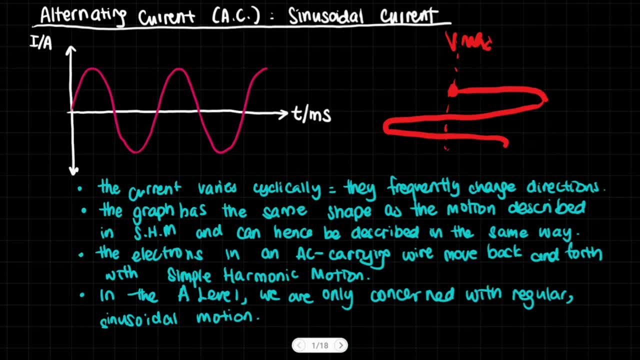 displacement of the object from the equilibrium position and it acts in in order to replace it back to the equilibrium, so it acts in the opposite direction. that's the displacement. that is exactly how the electrons are moving, because you keep going one way and then you keep changing, reversing. 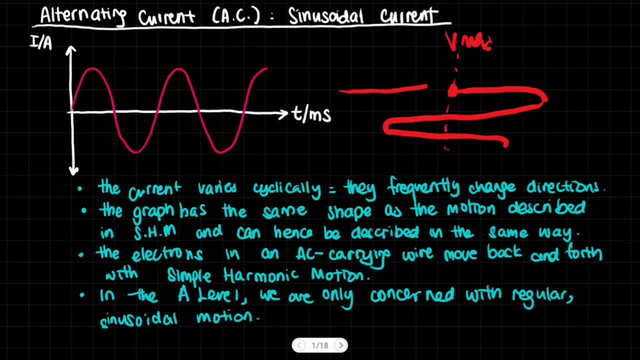 again and again. they don't really make progress. they just go here and they come back and this is this is what the electrons are doing inside that that wire. so let's take a look at the simple harmonic motion equations. these are the simple harmonic motion equations that you can also check. 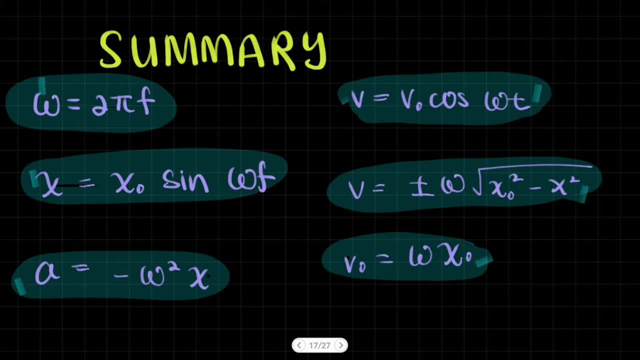 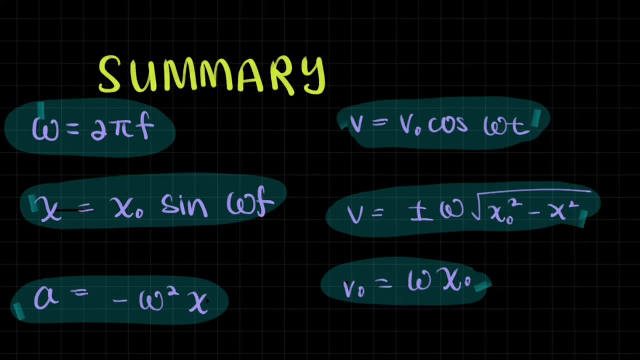 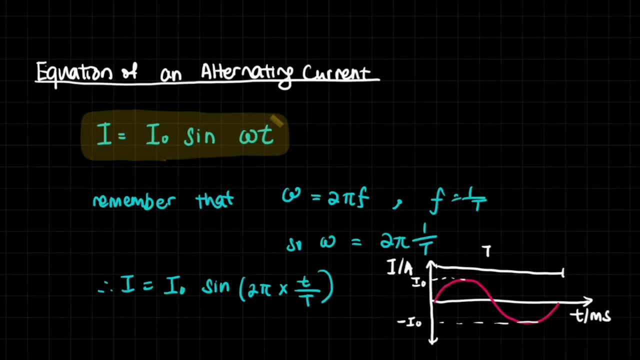 out in the video that i posted about all the equations in simple, harmonic motion. we have all of these: omega is two pi, frequency and stuff like that. we have all of this which can be useful, so check it out. so that's why we get you the equation of an alternating current, which is that the alternating current at any point in time. 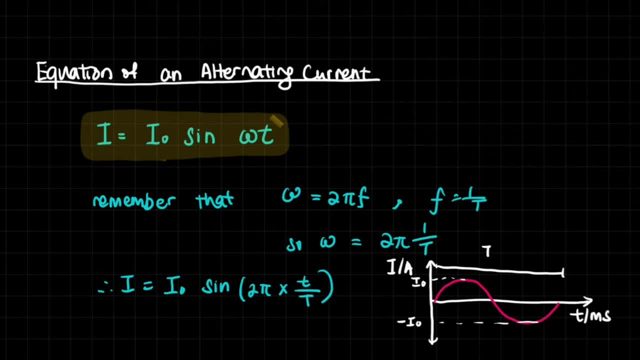 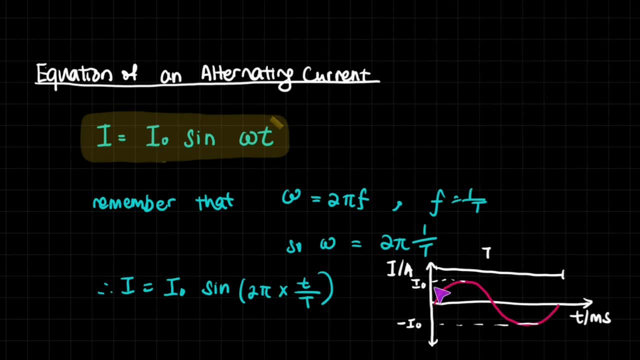 is i? o, sine, omega t, and this is just like the displacement right, and this is because it's in a sinusoidal form. now the i? o points towards the maximum current right, so you take the maximum current and then you times it by the sine to get whatever is the current at that point in time. 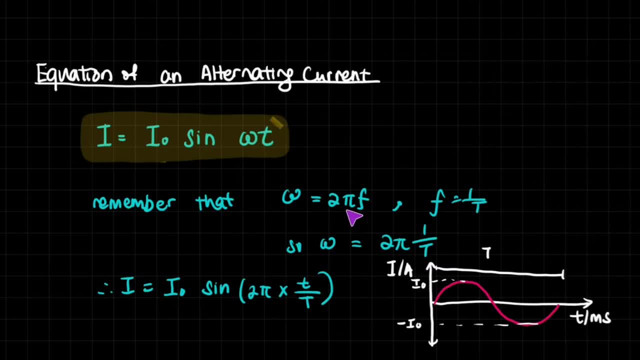 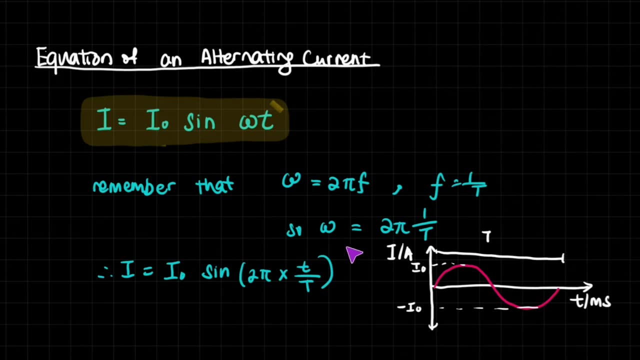 omega in this situation is actually two pi f, because this is not really circular motion. so you have to remember that omega is two pi f and f is one over the period. so if you substitute this inside, what you're essentially doing is omega is two pi one over t. 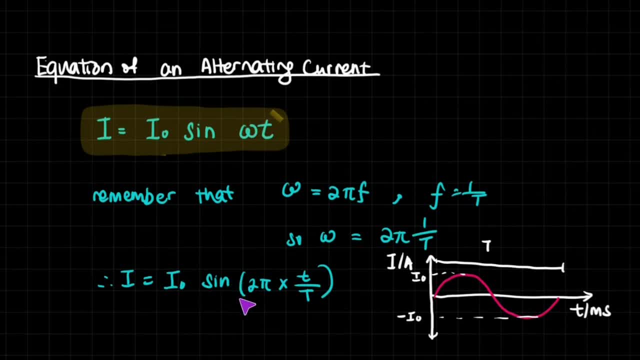 and that means if you times it in here, it's sine two pi times the time over the period. let's say that the period is three seconds, so you have this and that is three seconds and that is t. and let's say that you are currently trying to get. 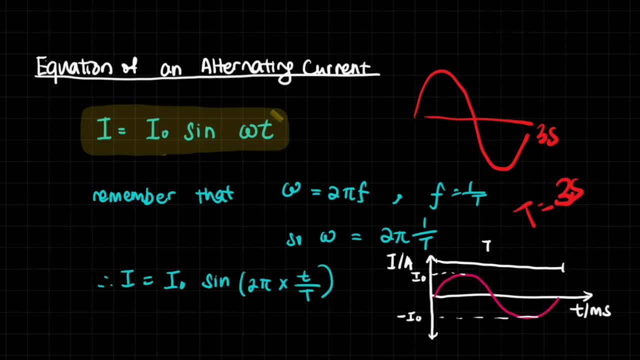 maybe you are at one second. then we have one second is around here, so you have t is one second. so you substitute that in. what you will basically get is one over three times two pi. so you're basically calculating how much fraction of that- the full cycle- you have gone, and there's just times about two pi, and then you get the final. 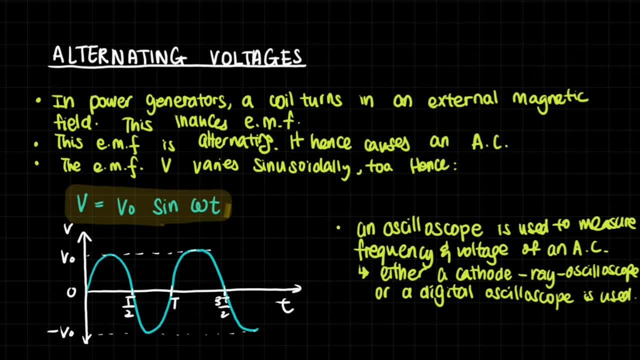 current. so current is always formed by the electromotive force or a voltage, and that's what drives the charges across. if you have an alternating current, then that means that there has to be an alternating voltage that is driving it. because the voltage keeps changing, the current also keeps changing its direction. now in power generators a coil turns in an external magnetic 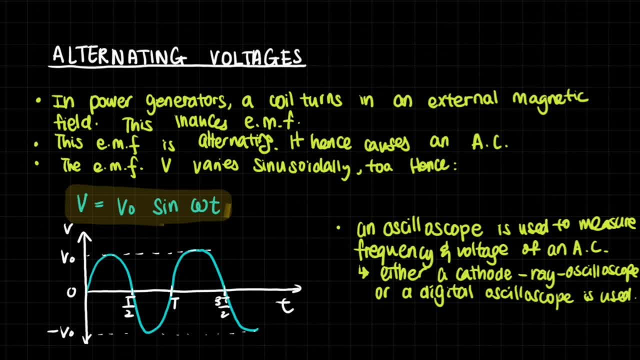 field and this induces emf. and so, as you have seen in the previous video, this induces emf that will continuously change direction in a sinusoidal way. so this electromotive force is also alternating and it causes an alternating current. the emf v varies sinusoidally as well. 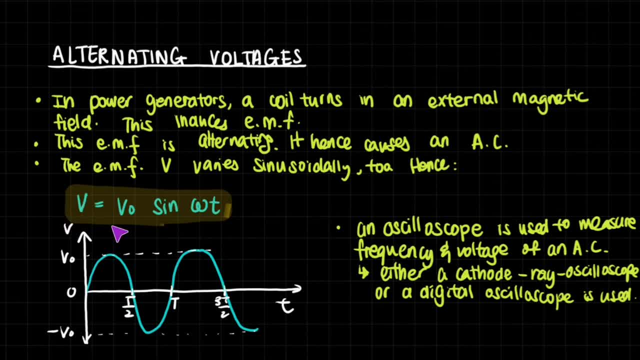 hence we can say that the velocity, the, the voltage as well, is the maximum voltage, vo sine omega t, just like the alternating current, and so this is also using the simple harmonic motion equations. an oscilloscope is used to measure frequency and the voltage of an alternating current, so you can either use 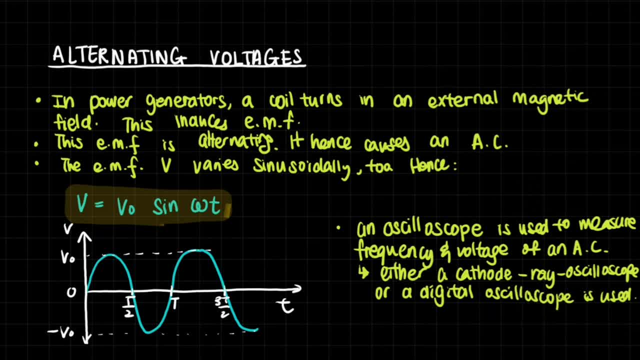 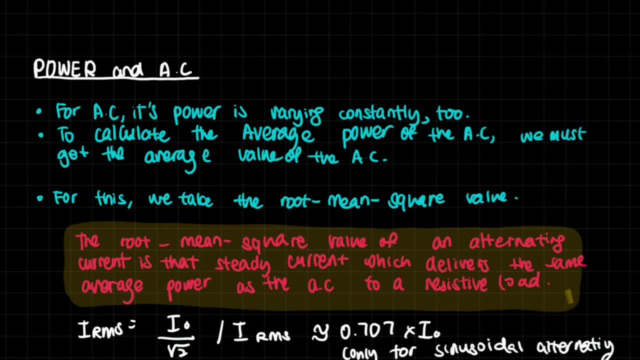 a cathode ray oscilloscope or a digital oscilloscope, and you have to be able to read these oscilloscopes, which i will make a video about in a while. so now let's talk about path power and alternating current, because you talked about the, the voltage. we've talked about the. 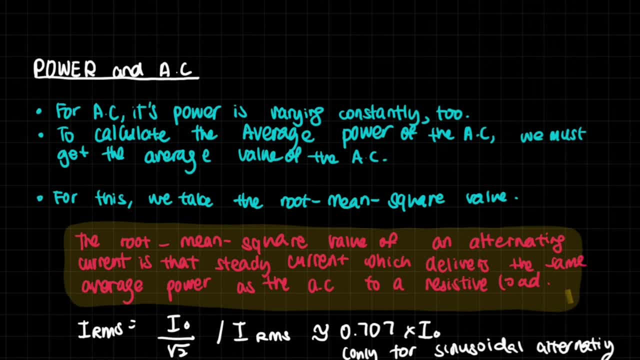 the current. so it makes sense to talk a little bit about power. and the question is: for alternating current, is the power that it supplies, the energy that it supplies, constant, or is it also changing? well, the answer is that it is actually changing constantly too. if you see some fluorescent lamps, 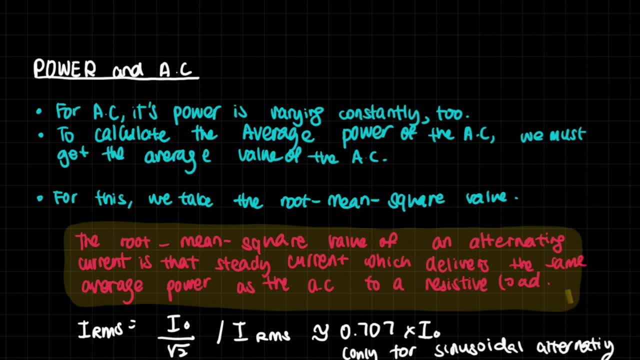 you will see that sometimes you can see a very quick flickering, and that's because the power that is supplied is also changing. however, it's very, very difficult for us to be able to deal with a a changing power. so what we are going to try and do is try to get the 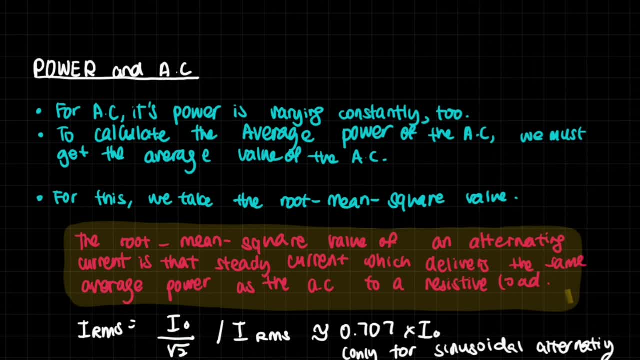 average power, the average energy per time, average energy dissipated per time. now, in order to get that, because we know that p equals iv, we need these values how we want to start, because we're going to say that p will be equal to iv. However, for us, these values keep changing because the alternating current and the alternating voltage are not the same. 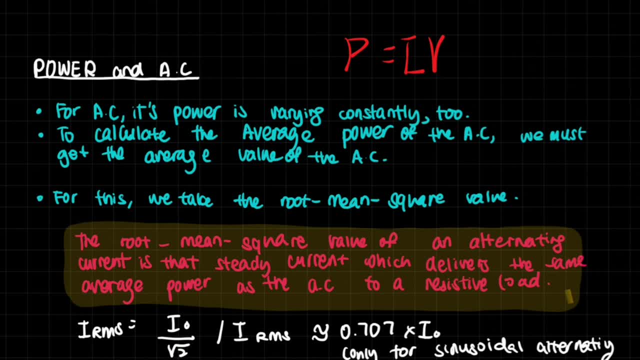 They don't stay constant. So what are we going to do? Well, we're going to get the average value of the alternating current and the average value of the velocity. This average value will stay constant and therefore we can use it in this equation. 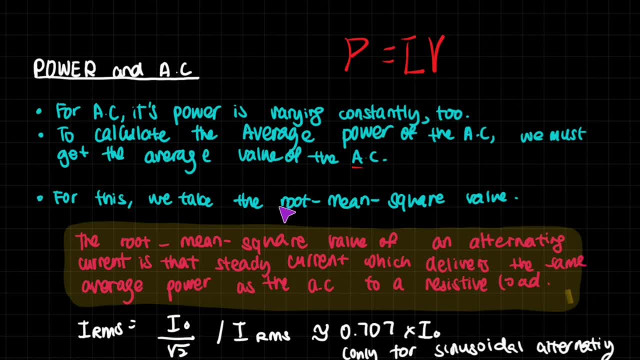 But getting this is a pretty difficult process. For this we take a look at the root mean square value. What is the root mean square value? The root mean square is a value of an alternating current, And this is the steady current which delivers the same average power as the alternating current to a resistance load. 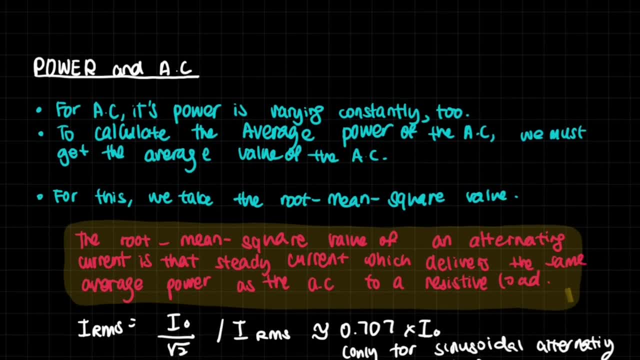 So a good way of picturing this is: we take a lamp, We take a light bulb or something like that, And then we hook it to a direct current, like direct current power supply, And then we take another one And we hook this lamp, which has to be the same power, like it has to have all the same ratings as this one to make it fair. 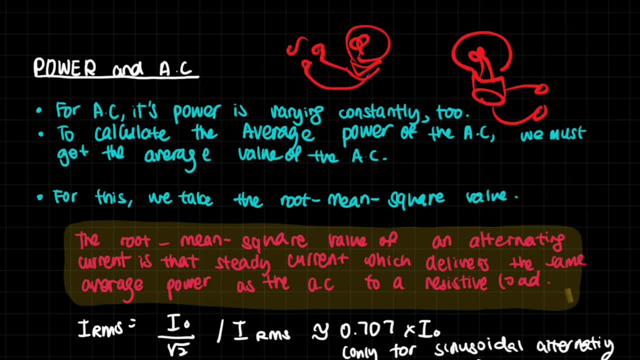 And we hook it to an alternating power supply. So when these two lamps are shining with equal brightness, then this means that the direct current value over here is equal to whatever alternating current maximum value is over here, And so if you try this out, then what you're getting is this: direct current is the root. 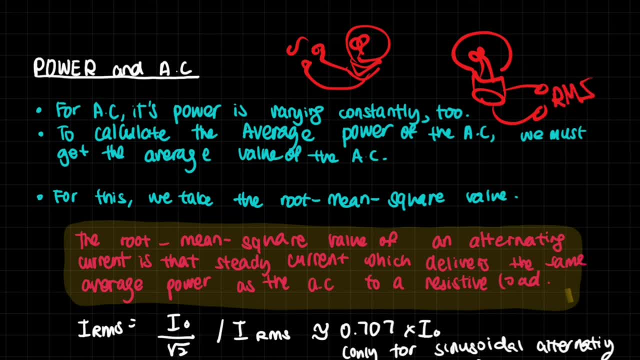 This is the root mean square of this alternating current. An average constant value that provides exactly the same on average as the alternating current And the root mean square is very important because the AC is constantly fluctuating. We have to use a special way to get this. 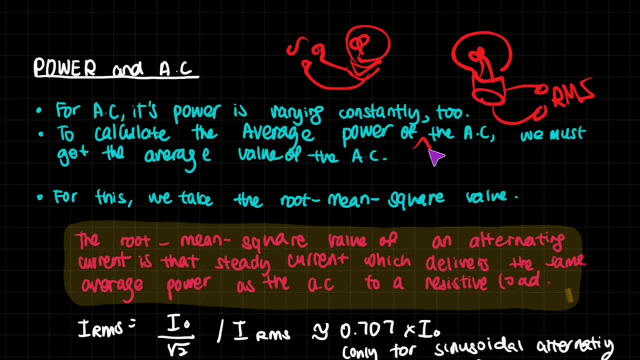 Because, as you know, this current is actually sinusoidal. The average value is you have to add everything together and then divide it. And if you add everything together over here- obviously because half of it is the negative value- you're just going to get zero. 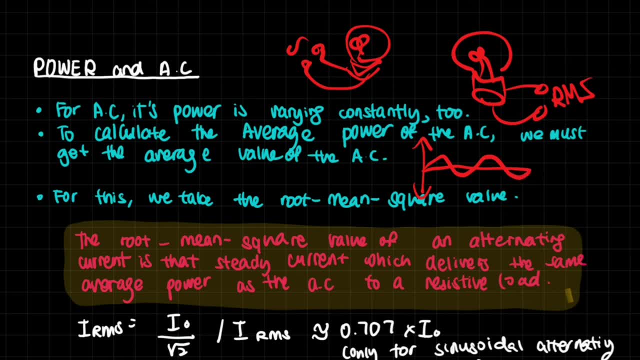 And so the mean has no meaning when it comes to this. So we have to use a special way to get it. Now. we derive the root mean square by squaring the alternating current like that: If you square it, it's going to become something like this: 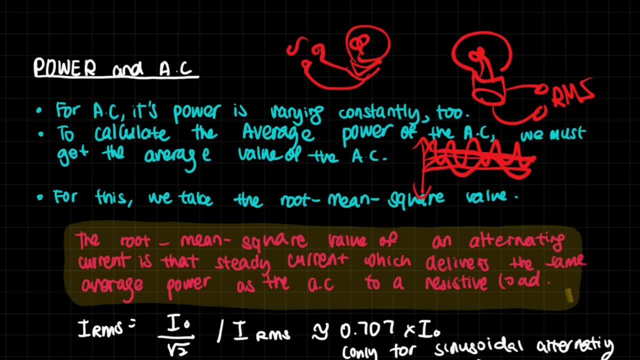 We take the mean which is the middle of that, and then we root it one more time So we put a square root off it so that you can cancel out this sort of thing. So eventually we get like a: take the current maximum and then you square that. 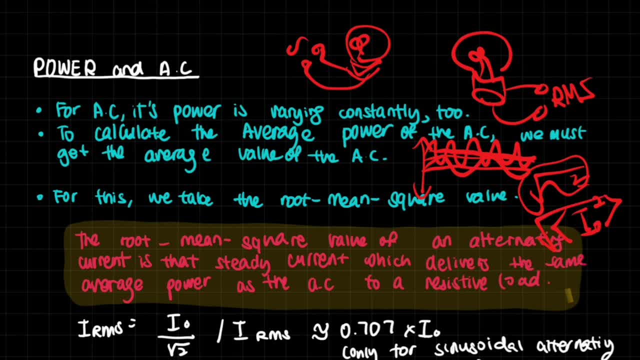 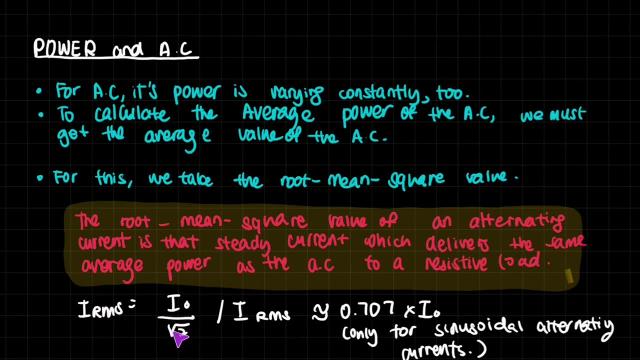 and then you take the average of that and then you square root it again, And so if you go through the entire process, which I will do in another video, you are going to finally get the answer that the root mean square is the maximum current divided by square root 2.. 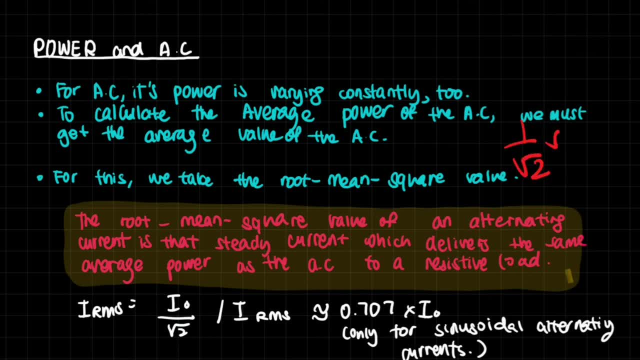 1 over square root 2 is, you know approximately, Approximately 0.707.. So if you put this you're going to get the root mean square is 0.707 times the maximum current. So just by knowing for a certain current what this is, I-O, you can get the root mean square.